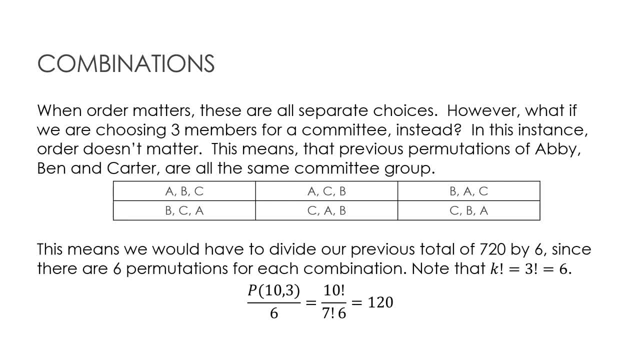 in that case order wouldn't matter And therefore everybody here in my little table it's exactly the same committee group, because it's a committee group that includes Abby, Ben and Carter. So essentially what happens is I have to divide my permutation group that I had before. 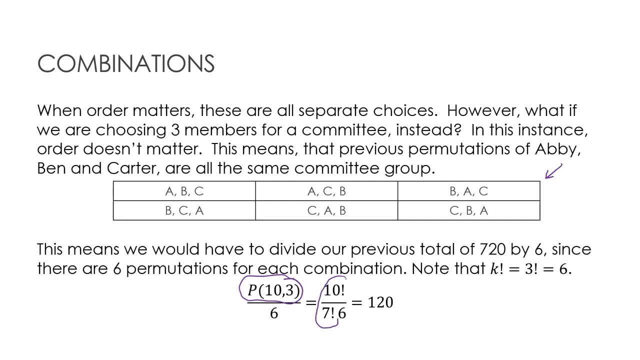 which was here including the 10 factorial, over 7 factorial, and I have to divide it by 6.. So where did 6 come from? Well, notice that k factorial k was 3.. k is 3 factorial. 3 times 2 times 1 is 6, that's where that little 6 came from. 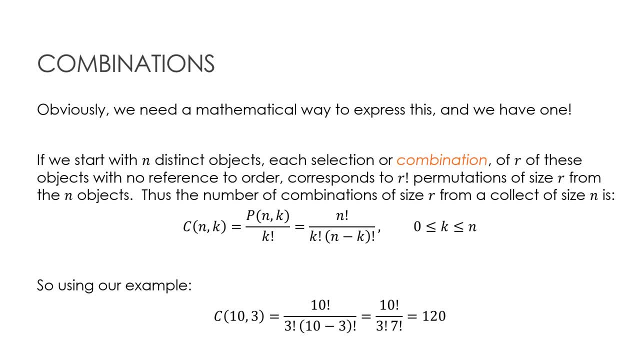 So obviously we need a mathematical way to express it, and of course we have one. If we are dealing with a combination instead of a permutation, a combination where order makes no difference, then we're going to find the permutation and we're going to divide it by k factorial. 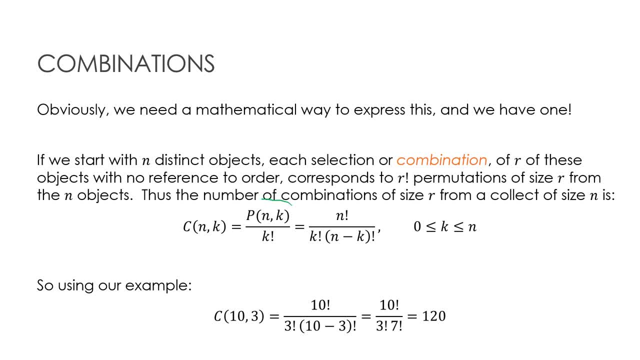 So if I take that to the next step and say: well, I know that this is actually n factorial over n minus k factorial, and then I have to divide that by k factorial, notice, all I'm doing is sticking another k factorial on the bottom. 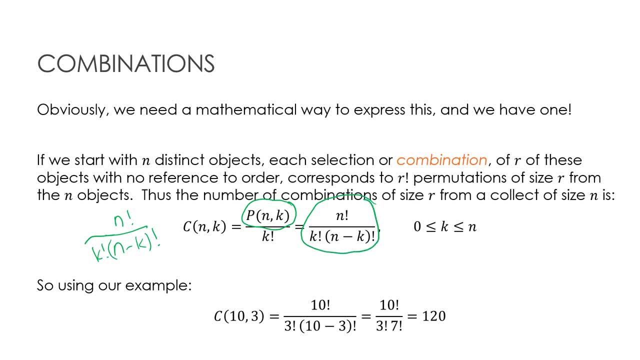 So this is my formula for a combination of n items choose k. So, using our example, again 10 choose 3.. This time for a committee rather than specific positions on the committee. It would be 10 factorial divided by 3 factorial, and then n minus k, which is 7 factorial. 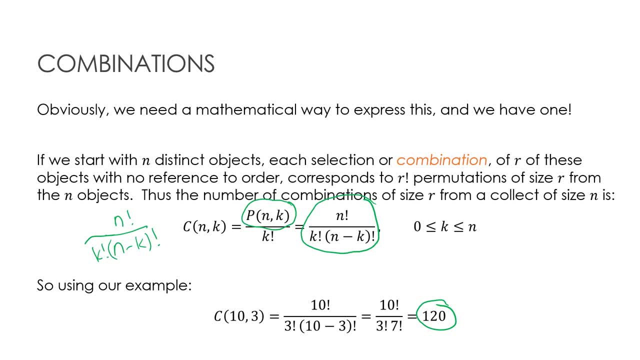 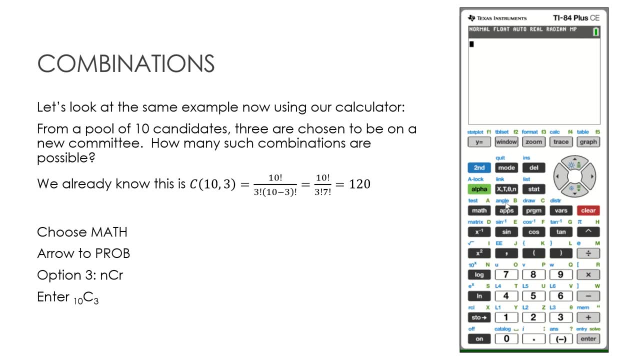 And that gives me the 120 that I already knew was the solution. Let's take a look at how to do this on our calculator. It's essentially the same process you're going to go through as before: Math arrow to probability. Previously, we chose npr. 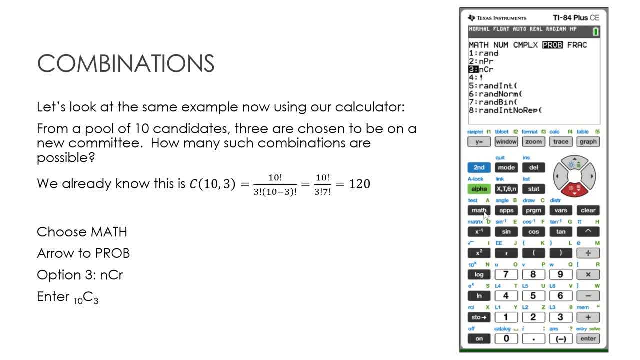 Now we're going to choose ncr for combination and again we're going to plug in 10, 3.. I should note, in case your calculator is a touch older than mine, that for some of these you will actually get something with a c. 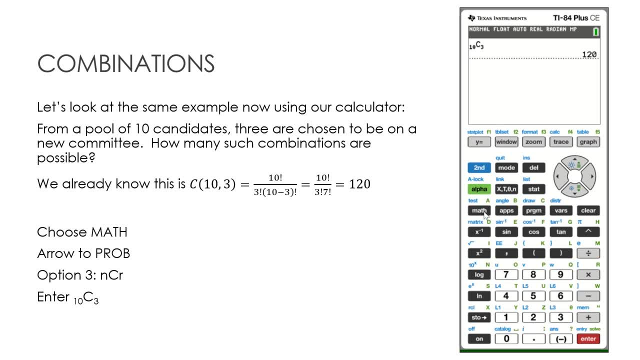 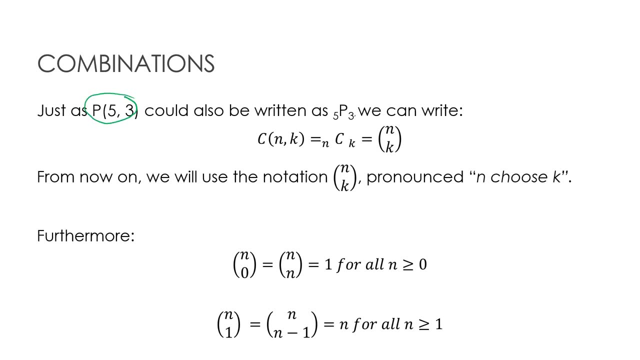 and then you'll have to enter in the parentheses 10,, 3,, just as we write it on our papers. So it kind of depends on the age or the style of your calculator. So when we dealt with permutations we said: okay, we can write it like this. 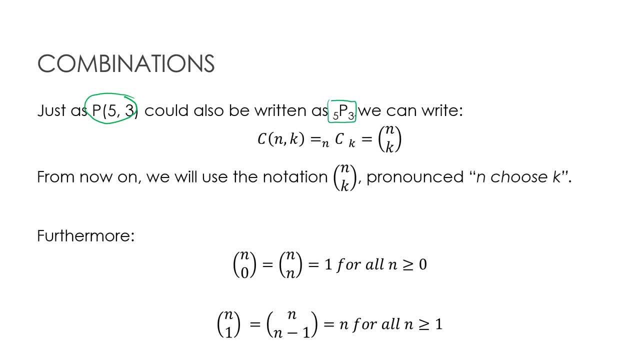 but then we put it in our calculator, it looked like this, And obviously we just saw on the last page that the same holds true for combinations. But what we haven't talked about before is this guy right here And from this point forward, this is how you're going to see these numbers. 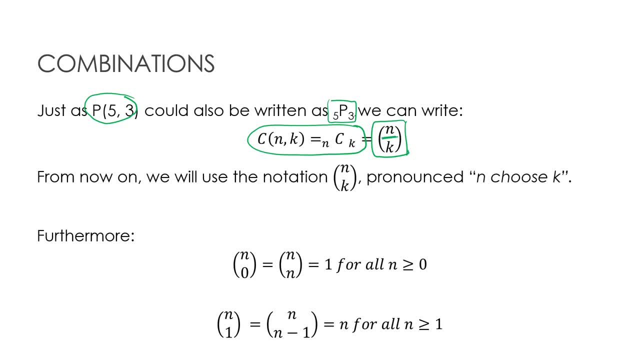 Notice: this is not a fraction. There's no fraction line in between, And this is n choose k. So when we have n choose k, it automatically means that it's a combination, not a permutation, in which case the order obviously does not matter. 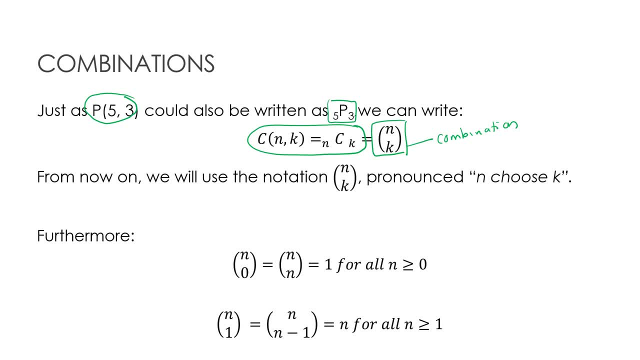 And then below I just have a couple of things that's important to understand- that if you have n, choose 0, so you have n objects and you're not choosing any. there's one way for that to happen and that's not to choose any of them. 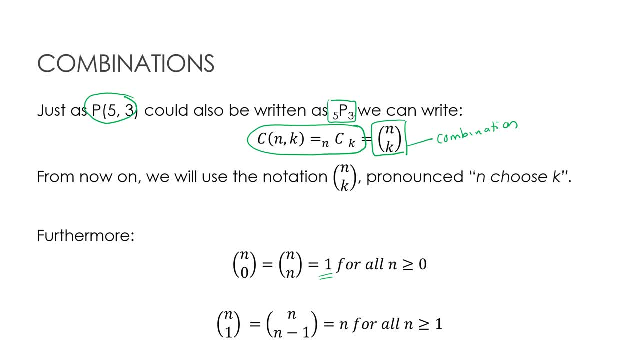 Or n choose n. if I have, say, 10 objects and I'm choosing all 10, because order doesn't matter, there's just one option for that. Another one that will come into play- actually quite often- is this guy. This will come into play when we start doing proofs and things. 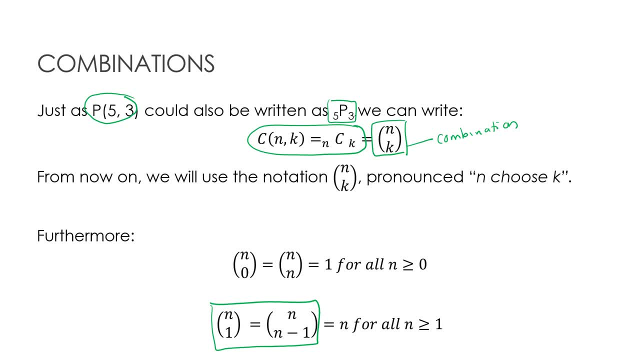 You might have to replace n choose 1 with n choose n minus 1.. And again it's the same idea. It's saying, if I'm choosing 1, then there's n different ways to do it, Or if I'm choosing essentially all but one thing. 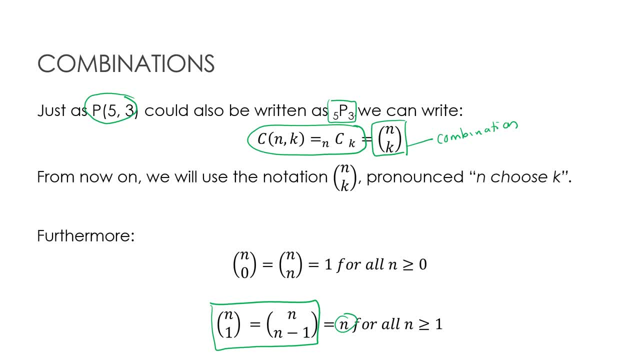 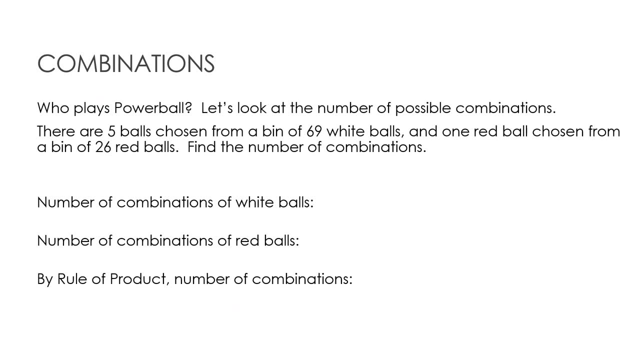 then there's n ways to do that as well, because you would be leaving one out each time. So let's take a look at Powerball. Who plays Powerball? A lot of people. Is it worthwhile? Well, let's take a look at how many combinations there are. 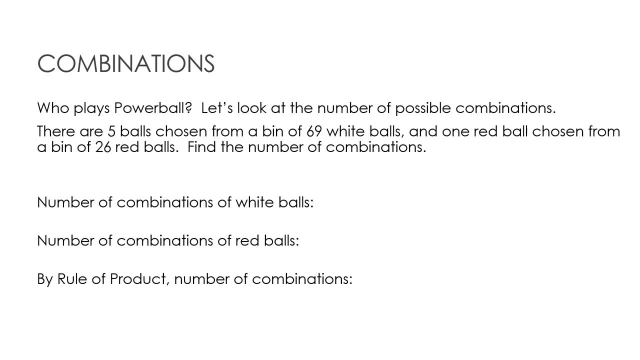 There are five balls chosen from a bin of 69 white balls and one red ball chosen from a bin of 26 red balls. Find the number of combinations. So let's start with the number of white balls. There are 69 white balls. 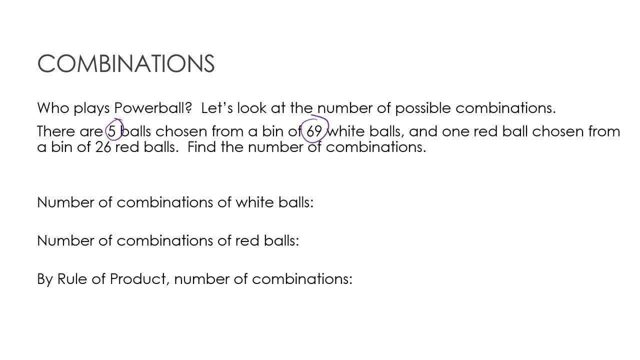 How many of those are we choosing? We're going to choose five of those. So 69, choose 5.. Now notice, I haven't found that as a raw value yet. That's just 69 choose 5.. Same thing for red balls. 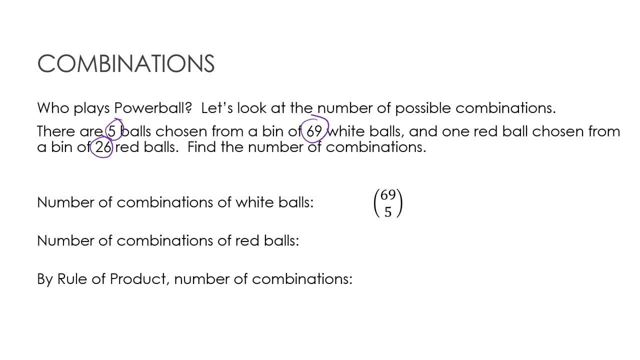 How many red balls are there? 26.. How many are we choosing? Just one: 26 choose 1.. Because I'm choosing five white balls and one red ball. that means we're using the rule of product, We're multiplying. 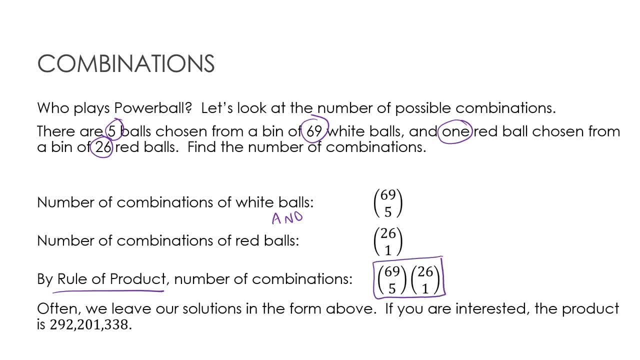 And so I would have 69: choose 5 times 26, choose 1.. Now, if I use the product rule, this is how many different options there are. How many of those options are winners? 1., 2., 3.. 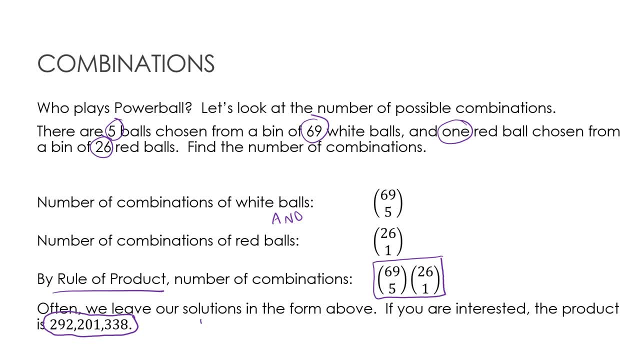 4., 5., 6., 7., 8., 9., 10., 11., 12., 12., 13., 14., 15., 16., 17., 18. 19.. 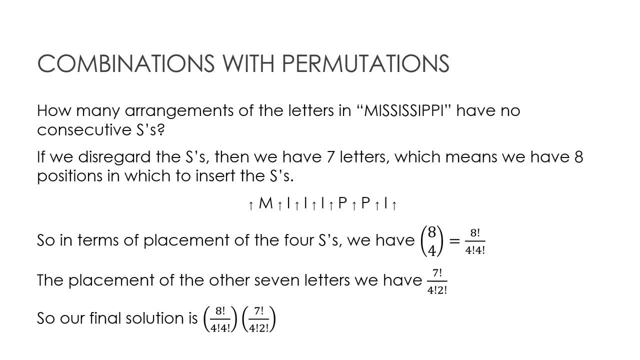 20., 21., 22., 23., 24., 25., 26., 27., 28., 29., 30., 31., 32., 33., 34., 35., 36.. 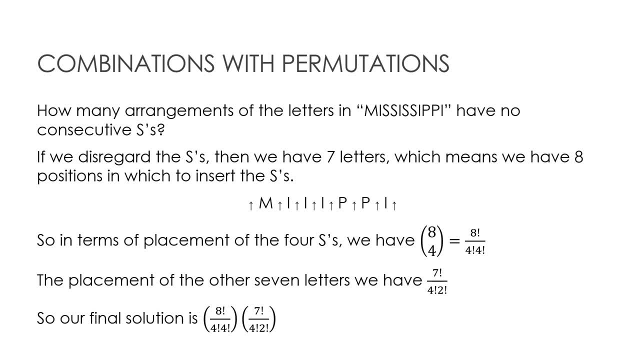 36., 37., 38., 39., 40., 41., 42., 42., 43., 44., 45., 46., 46., 47., 48., 49., 50.. 51., 52., 53., 53., 54., 55., 56., 57., 58., 59., 60., 61., 62., 63., 62., 63., 64.. 65., 66., 67., 68., 69., 69., 70., 71., 72., 72., 73., 73., 74., 74., 75., 76., 77.. 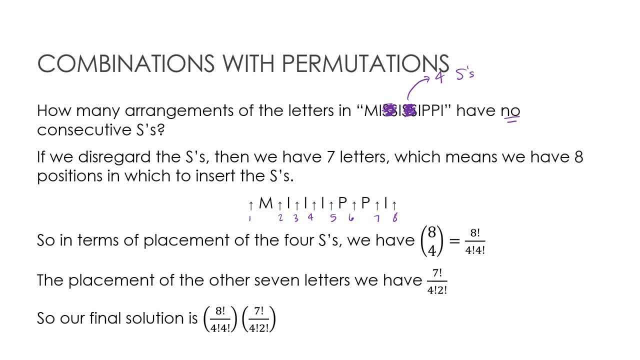 78., 79., 80., 80., 81., 82., 83., 84., 85., 86., 87., 88., 89., 90., 91., 92., 92.. 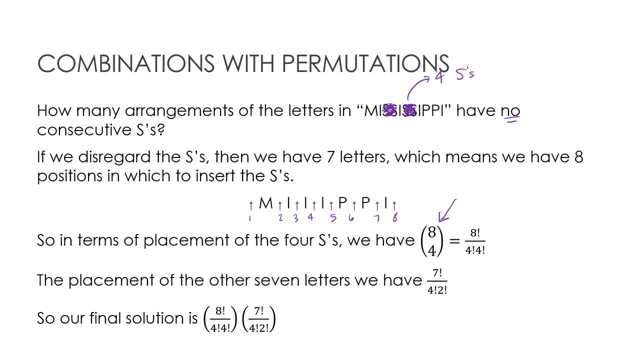 93., 93., 94., 94., 95., 95., 96., 96., 97., 97., 98., 98., 99., 100., 100., 100. 100.. 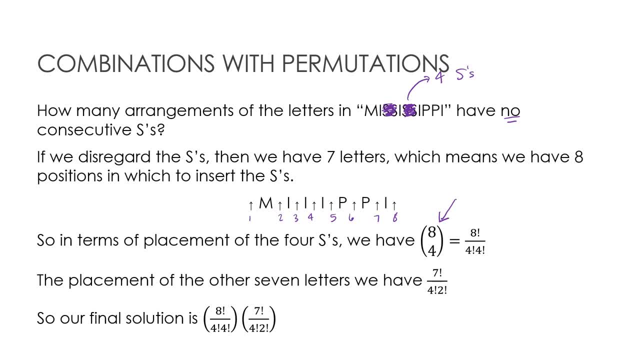 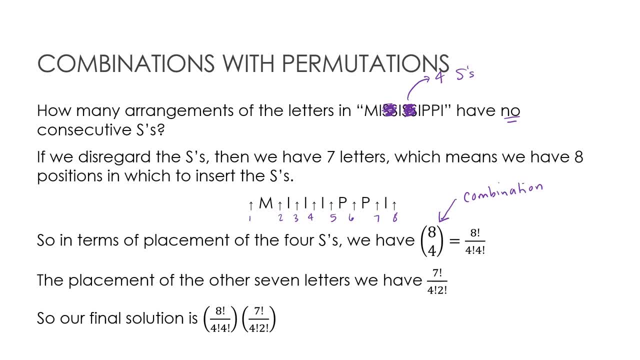 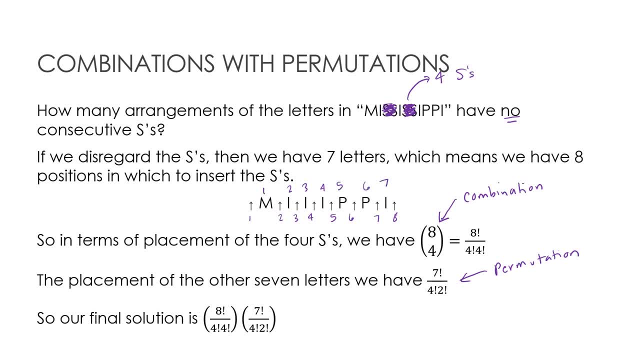 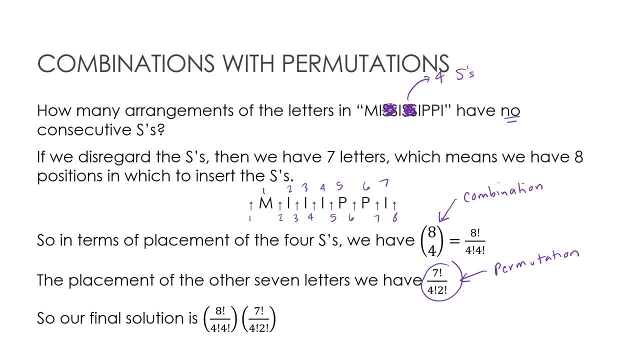 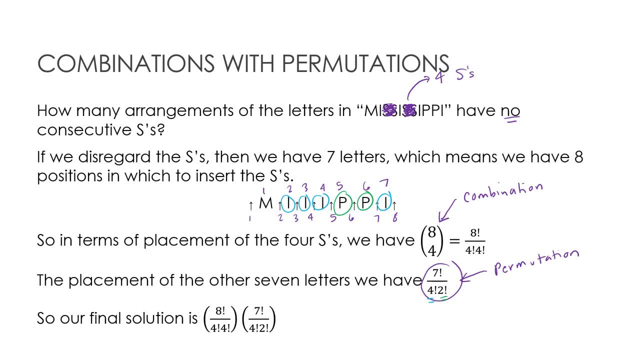 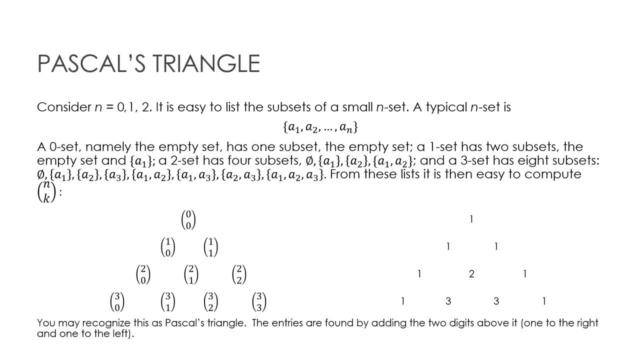 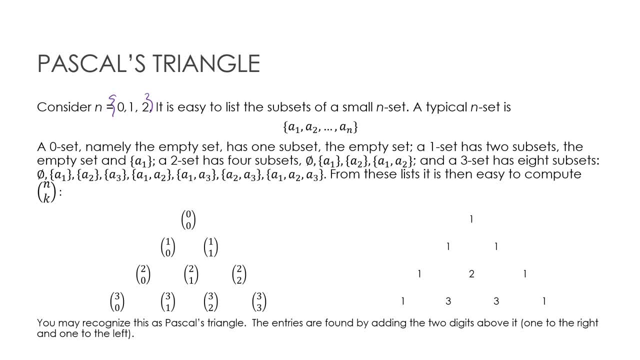 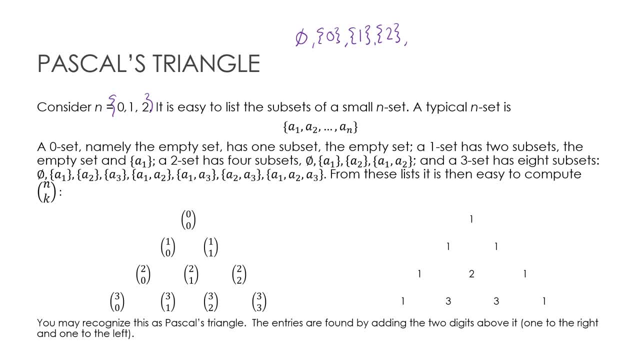 one element. I could have subsets with two elements, so 0, 1,, 0, 2, or 1, 2.. Or I could have a set with three elements, which would, of course, be the set that I started with. 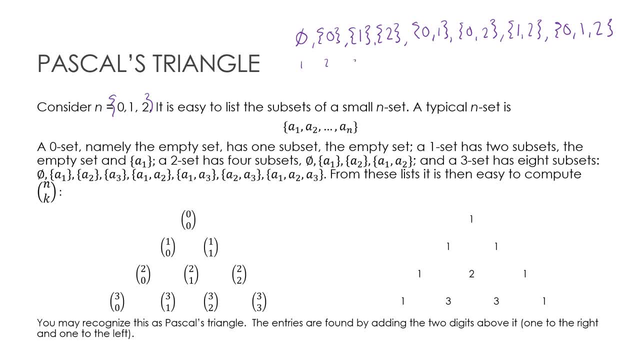 0,, 1, and 2.. So I have 1,, 2,, 3,, 4,, 5,, 6,, 7, 8 total subsets. So let's say I didn't have just three tiny little elements in a set and I had 100. 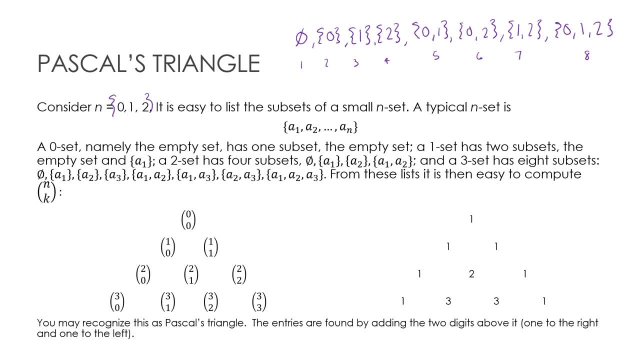 Well, how would I then determine what I'm dealing with? Well, this is where Pascal's triangle comes into play. So let's say I have a 0 set, which is an empty set that has one subset, which is, of course, the empty set. Let's say I have a 1 set, meaning there's only one element. 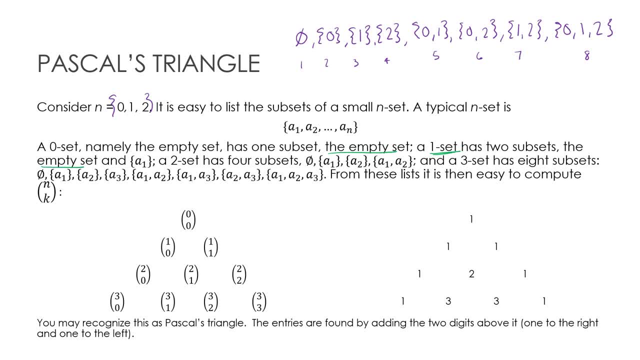 then it has two subsets: the empty set and the only element in the set. Now, before I continue, let's look down here. This would be for my empty set: 0, choose 0.. Okay, this would be for my 1 set. I have one element and I can either choose 0. 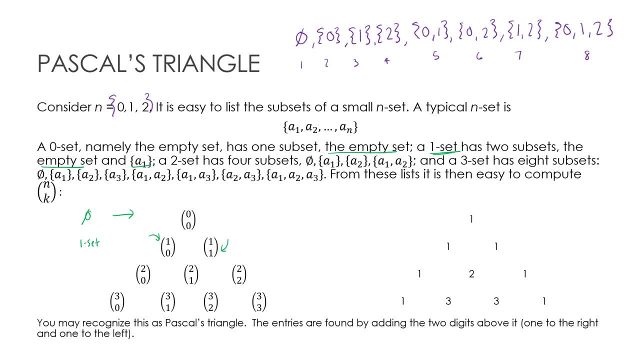 or I can choose 1,, either 1,, and that's what I've listed so far. So now let's take a look at my two sets, which is that I have four subsets. I have the empty set, which means I choose 0,, I can choose 1,, or I can choose 2.. 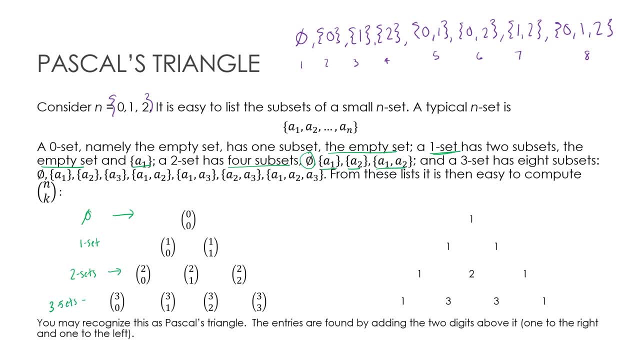 And then I have my three sets. Well, we already went through this one above up here, because that was the three set. I can choose 0,, I can choose 1,, I can choose 2, or I can choose 3.. Now this Pascal's triangle. 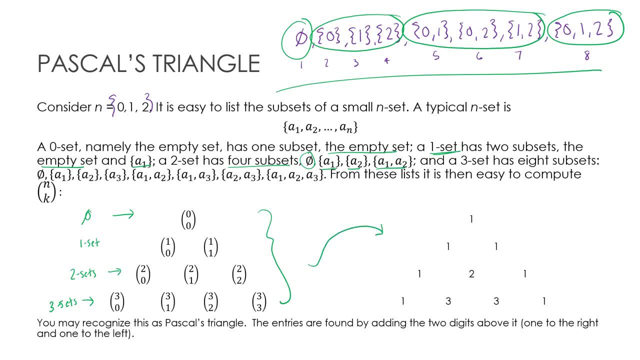 translates to these values: 0s- choose 0 is 1, 1- choose 0 is 1,, 1- choose 1, etc. Now, what do these pertain to? Well, if you'll look at this row, which we looked at in more detail, I had one. 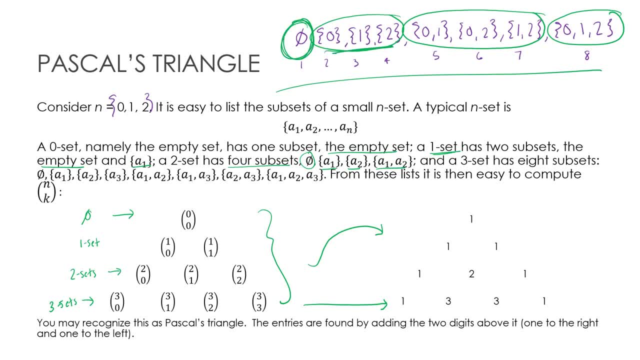 set that included nothing. I had three sets that included 1.. I had three sets that included 2, 3- choose 2.. And I had one set that included 3, 3- choose 3.. Again, why is this helpful? Well, we can also continue this triangle. 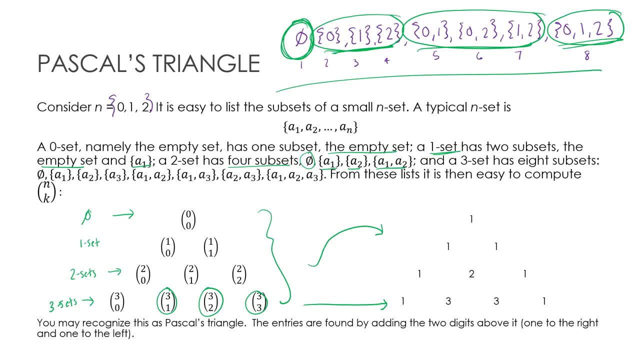 by adding the two digits above it, 1 to the right and 1 to the left. So, if you'll notice, these two add up to 3,, these two add up to 3, this plus nothing adds to 1, we get the idea. 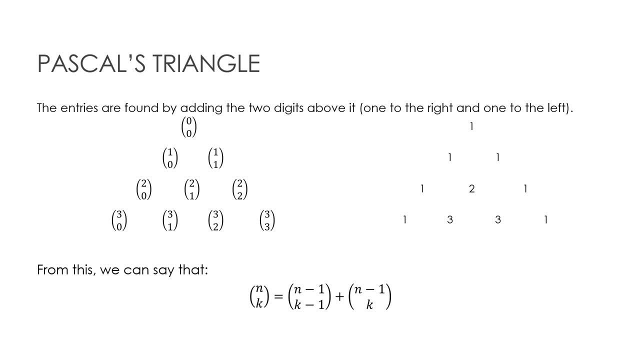 Now, mathematically, what does it mean when I say that I can take 1 to the left and 1 to the right and add them together to get 2, or to take these two to add them together to get 3, or these two to get 3?? 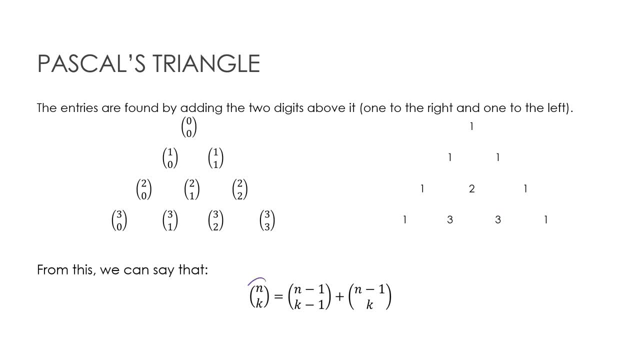 Well, essentially what it means is that n choose k, say this guy can be found by n minus 1 choose k. so this n would be 3.. This would be n equals 2.. So this is saying take 1 before it, which means the row before it. 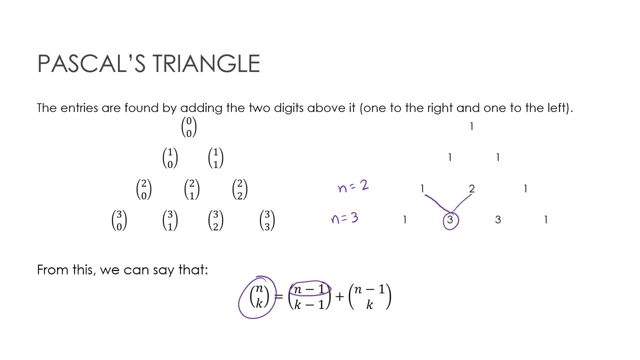 and then do k minus 1, and then do k. Now again, that might seem silly, but this is going to come into play all over the place. So this is one of those formulas that you write down on whichever special page you have to write down your special. 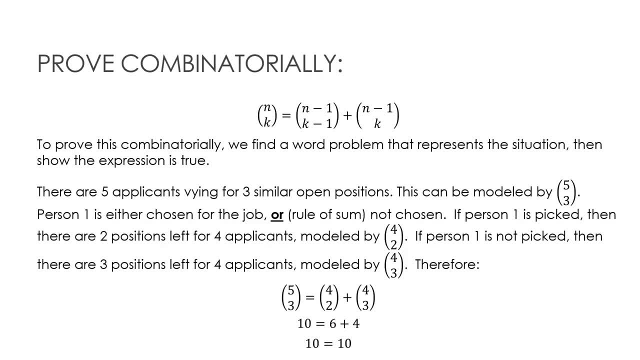 formulas on that you never want to forget. So in this course, we're going to do a lot of proof, and I'll often ask you to do one of two different kinds of proof. Prove combinatorially is something that you have never done before, So we're going to take our time on this one To prove this. 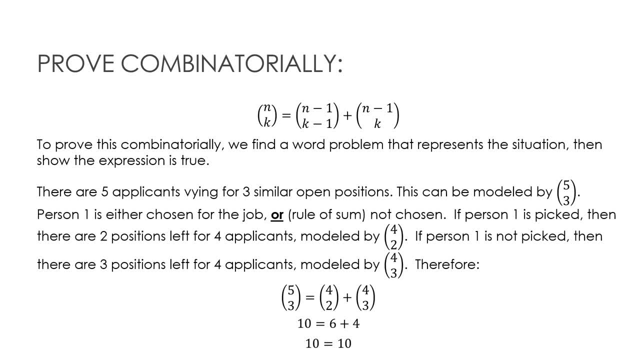 combinatorially. essentially, what we're going to do is we're going to find a word problem that represents the situation, then show the expression is true. So this is not like an algebraic proof and I'll show you that one in a little bit. Essentially, I want to think about how I could. 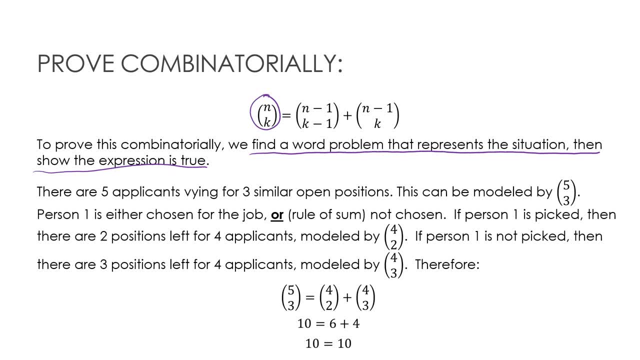 model and choose k and make it make sense for this formula. So explain it in a way that makes sense in a story problem. essentially So. for instance, here's one example. Let's say there are five applicants Vying for three similar positions. So notice, instead of choosing n and k, I've chosen to use 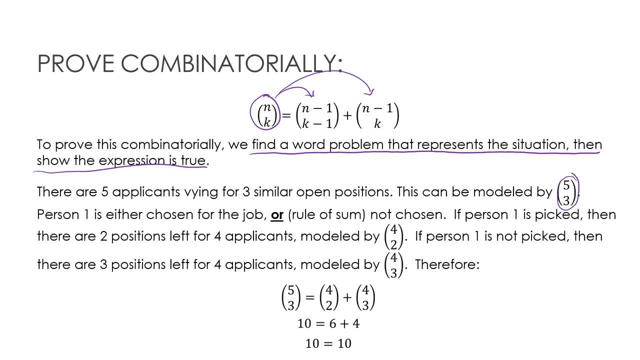 five and three, So five choose three. Now, I know that I can mathematically find five choose three, but that's not what I'm concerned about. My concern is: how do I make this part of the expression make sense in terms of that I have five applicants vying for three similar open positions. 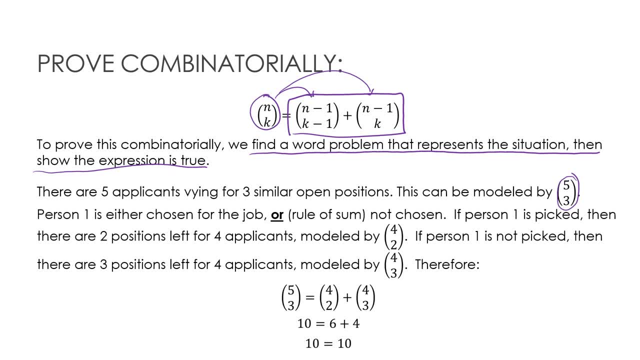 So I can say person one is either chosen for the job or rule of sum because it's or or not chosen. So if person one is picked, there are two open positions left for four applicants modeled by four. choose two. If person one is not picked, then there are three positions left for four applicants modeled. 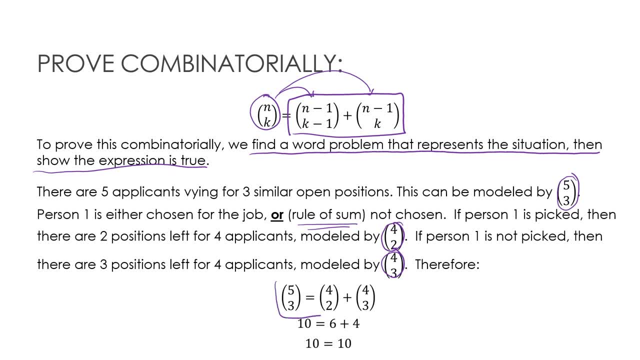 by four choose three. So let's take a look. Is it true, then, what I just said in the story problem that says five choose three is the same as one minus that and one minus k. I'm sorry, k minus one, n minus one, k minus one, which would 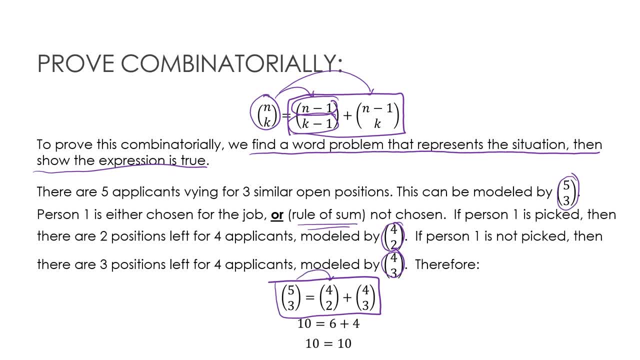 be the four choose two and then n minus one k four choose three. So in my story problem that seems to make sense. If person one is chosen, then there's only two positions left for the four people left over. If person one is not chosen, there's three positions left for the four people left over. 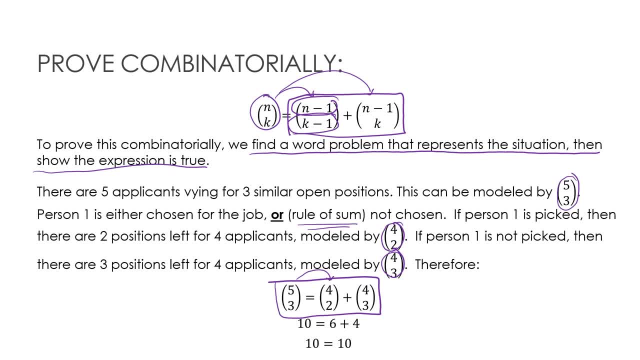 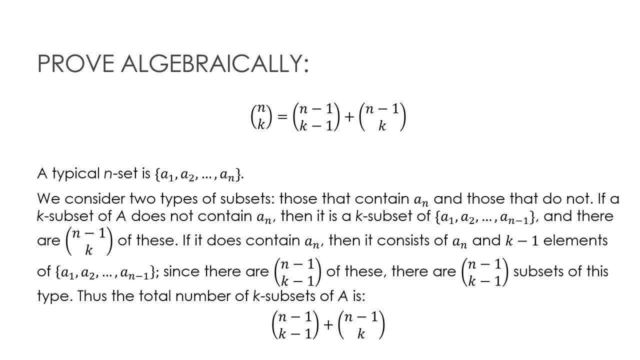 So if I do five, choose three again, you can use your calculator for that- I get ten. Four choose two is six. Four choose three is four. Notice, ten equals ten. So I've proven this combinatorially. Let's take a look at that exact same expression and now prove it algebraically. So now instead. 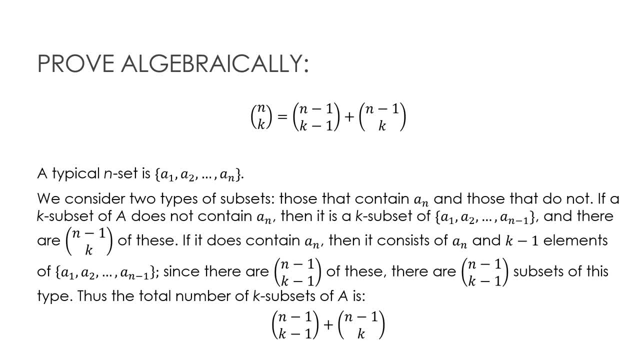 of making up a fun little story problem about people vying for a job, I'm saying let's look at the math here. So this is going to be mathier than our combinatorial proof. So we're saying we have a typical n set, N set being that there are n elements in the set, and we consider two types of 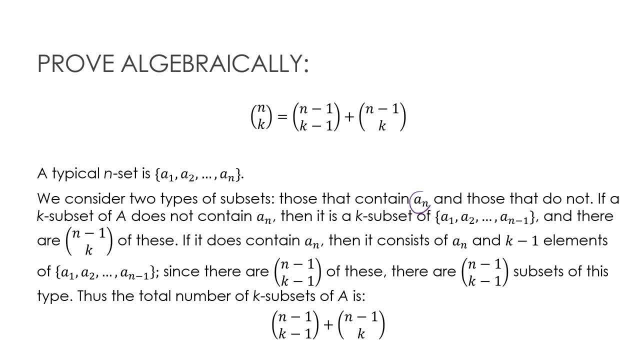 subsets: Those that contain a sub n, which is whatever our last guy is, and I could have said a sub one, two, it doesn't matter- and those that do not. So if a k subset of a does not contain a sub n, then it is a k subset of a sub one, a sub two, etc. all the way to a sub n minus one. and there 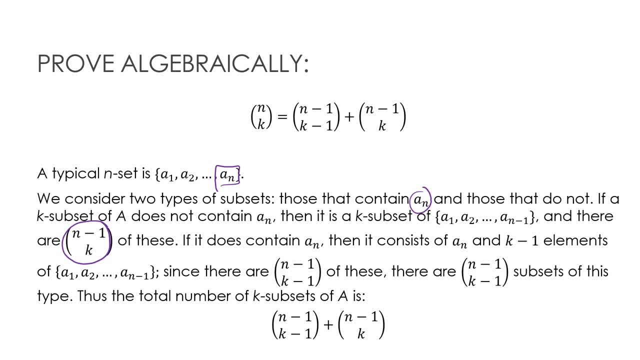 are n minus one. choose k of those, because again, it's a k subset. If it does contain a sub n, then it consists of a sub n and not k elements, but k minus one element, because, I've already said, n is a sub n, so it's going to be a sub one plus k minus one. So instead of k, it's k minus one. 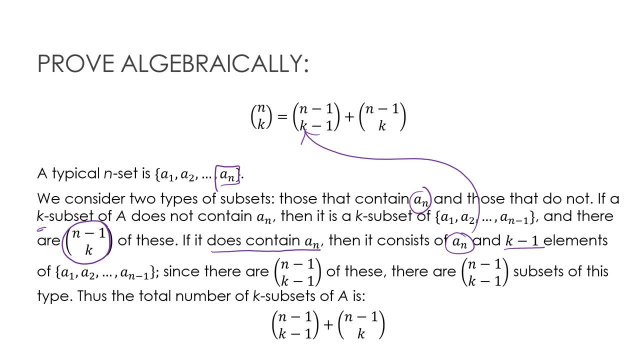 So that's this guy. Since there are n minus one choose k minus one of these and there are n minus one choose k of the other subsets, my total number of subsets looks like this: So, essentially, what I've done is I've said: if I have n, choose k, which is where I started and I break it into. 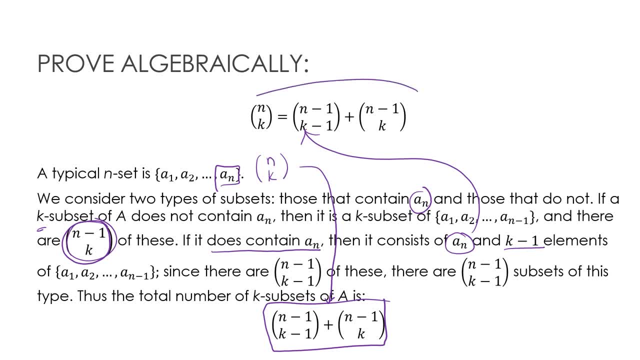 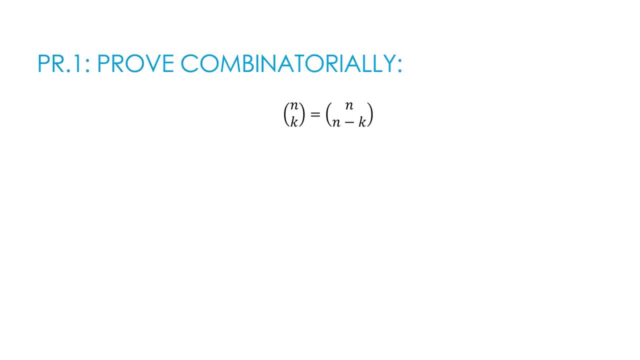 subsets- those are the two subsets that I get- which proves this algebraically? Here is another combinatorial expression that I would like you to prove is true: that n choose k is the same as n choose n minus k. So prove this, not algebraically. 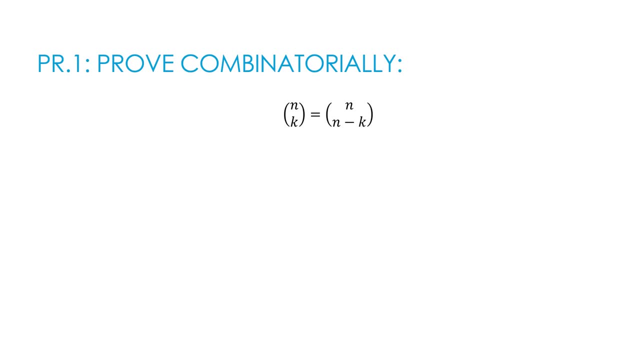 but prove this combinatorially. When you are ready, press play to see how you did So. keep in mind that you could have described this differently than I do. I just went straight for the five applicants vying for three similar positions again, and what I can say is: five choose. 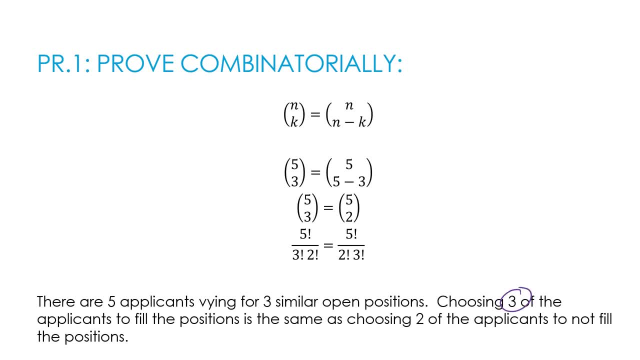 three is me choosing three of the applicants to fill the positions and n choose n minus k would be five choose two, which is essentially me saying I'm choosing two applicants that will not fill the position. And then I'm also showing here that if I took five choose three, I would get five factorial over. 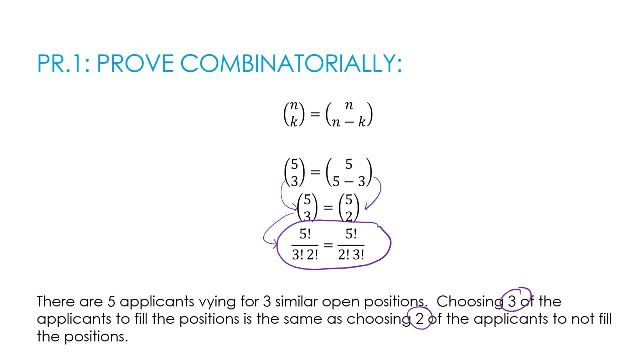 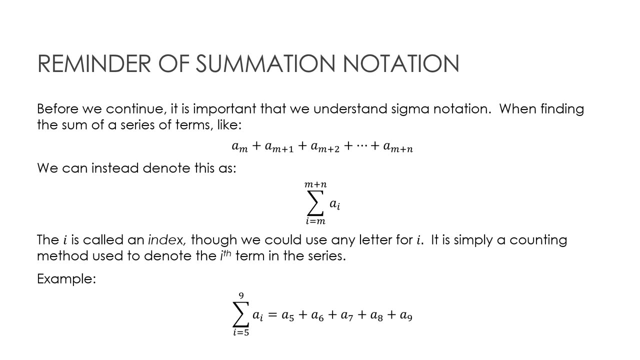 three factorial, two factorial. If I choose five, choose two. notice I get the same thing. It's a little bit different order, but we know that that doesn't matter with multiplication. So before we continue, let's just review sigma notation very quickly. When finding the sum of 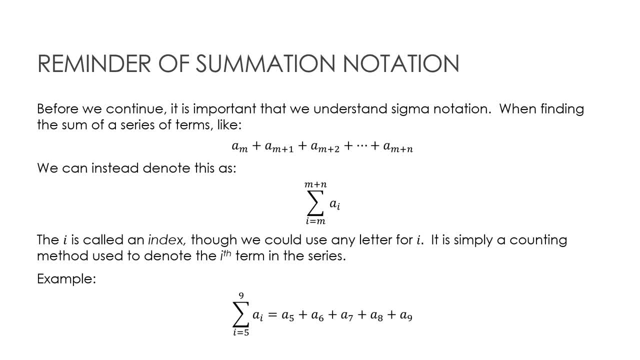 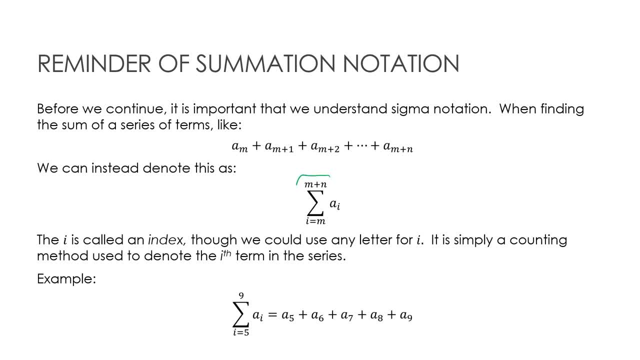 which is the summation notation. that says: take the summation of all values starting at m through m plus n, where i is being replaced by m through m plus n. essentially, The i is called the index and we can use different letters for it. 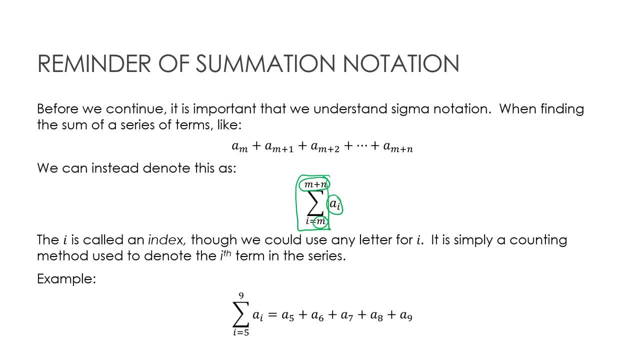 For i often j or k, but most of the time you will see it as an i, And again it's simply a method to denote the ith item in a series. So, for instance, if I said i equals five through nine, so find the. 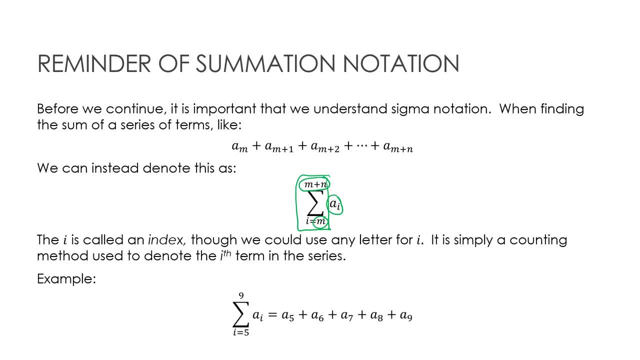 summation from five to nine of a sub i. that would mean a sub five plus a sub six plus a sub seven, a eight, a nine. And again, what are those numbers? I have no idea because I didn't. I didn't give you the series. So if I gave you the series and let's say it was just my counting- 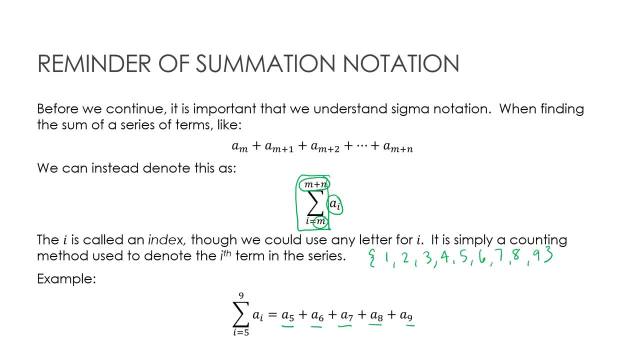 numbers. then you could say a sub five, so this is a sub one, this is a two. the second item, this is a three, a four, a five, but they don't always match up like that, So it could be that. 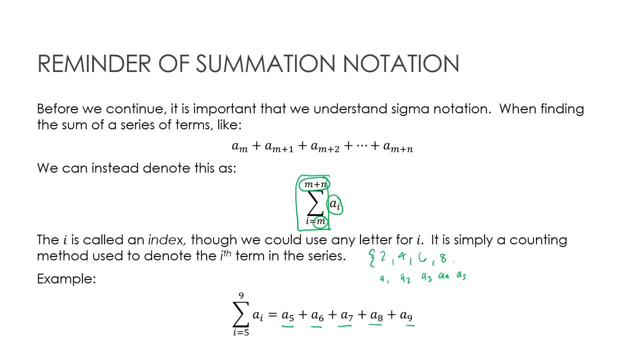 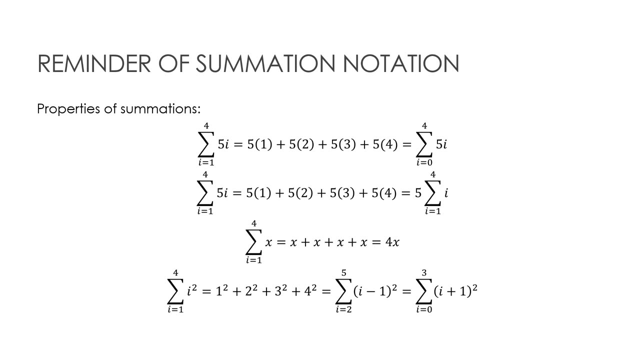 these numbers were two, four, six, eight, ten, twelve. you get the idea. So this is just saying j equals three times two times j, j and j plus j equals nine. Facebook cuad pra Een. What you can do to read a bunch of the other reasons I've mentioned earlier is: and let's 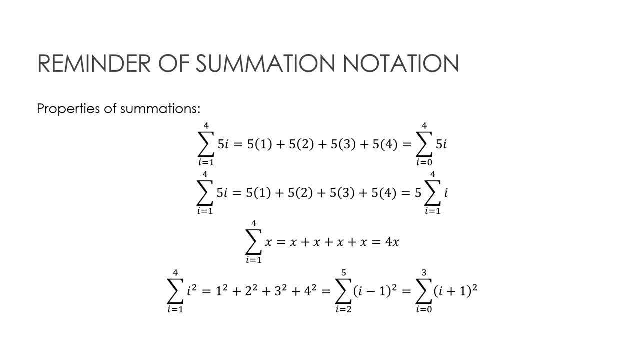 say, you can read or you have information about someone, depending on who it is. but you know what, when you're thinking about, oh, this is who it is, or this is the one who did that, or this is the one that did it, you're gonna need to start that information generally. 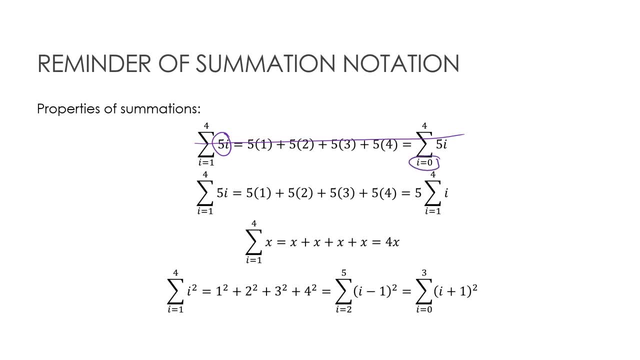 to make it work. It's not going to change anything if I include the 0, because 5 times 0 is 0, and so it's not going to change my sum at all. So that one's kind of silly and honestly, you don't come into contact with it that much. 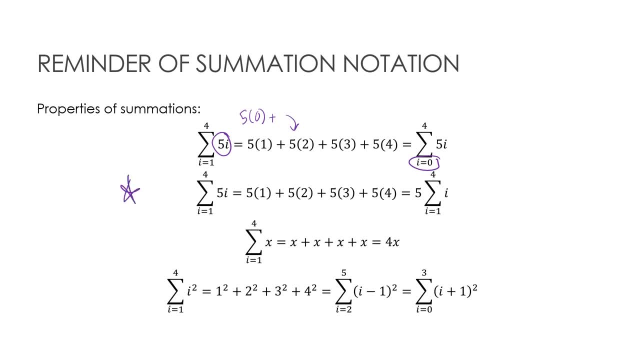 The second one you use all of the time and this basically says: if you've got a number like 5, it's okay to pop it to the outside. because essentially, what would happen if I took the summation 5 times the summation of this? it would be 5 times 1 plus 2 plus. 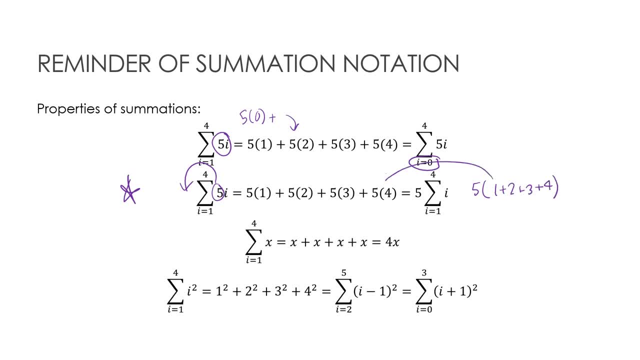 3 plus 4, and it would give me the exact same thing that I had here, This one. you also use a lot If you don't have an i in what you're finding the sum of essentially each time you use the index. this is the first, second, third, fourth: all you're doing is just writing x. 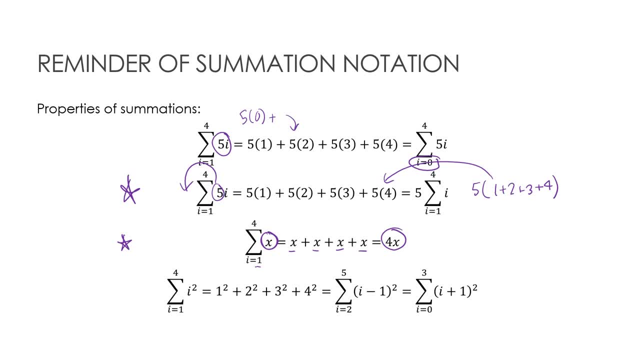 again. So my solution, if I wanted to simplify, is 4x. And the last one. this one's for those tricky examples, because sometimes we have to be a little bit tricky with our math. If I'm finding the summation of i squared, I can alter those limits: the lower end and 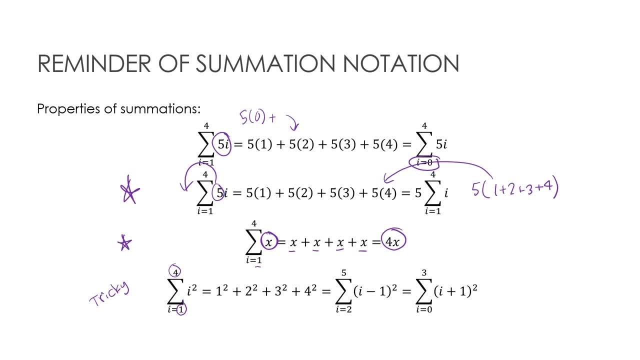 upper end of my index to adjust to a certain situation. So here I'm taking notice, I've added one here, and added one here Because here I subtracted one from i, So still this would be 2 minus 1 squared, which would be 1 squared. 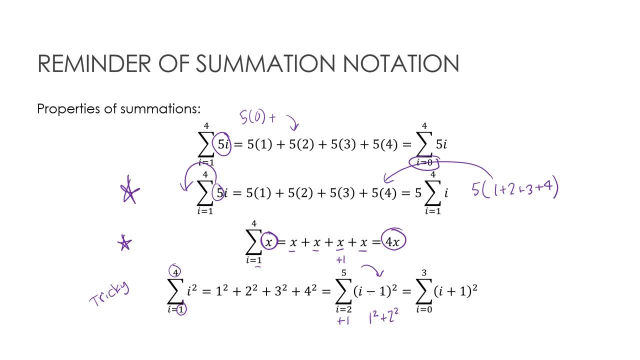 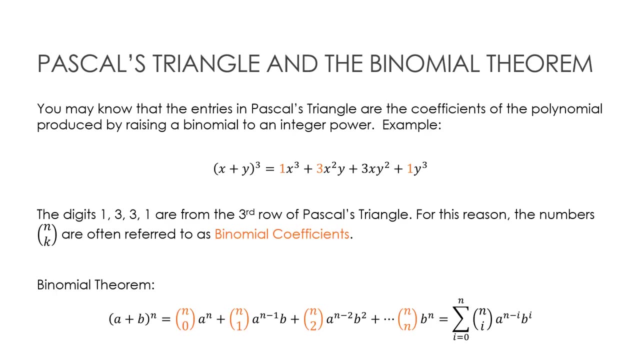 And then 3 minus 1 squared, which would be 2 squared. Same thing if I go in the other direction. Here I subtracted one and subtracted one, because here I added one and it would be the same thing. So we've looked at quite a bit so far and it hasn't necessarily all melded together. 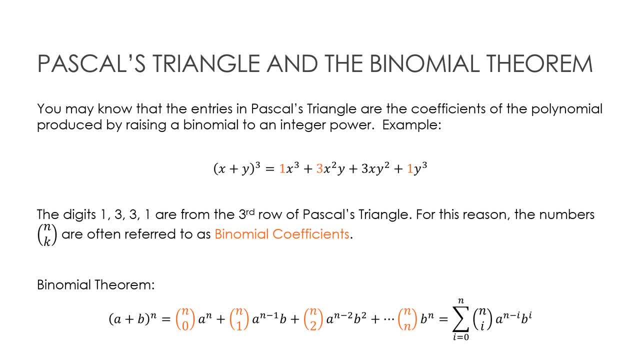 yet, And this, hopefully, will meld Everything that we've talked about in this section 1.3, together. So we've talked about Pascal's triangle, We've talked about how to write a binomial value like 4 choose 2, n choose k, etc. 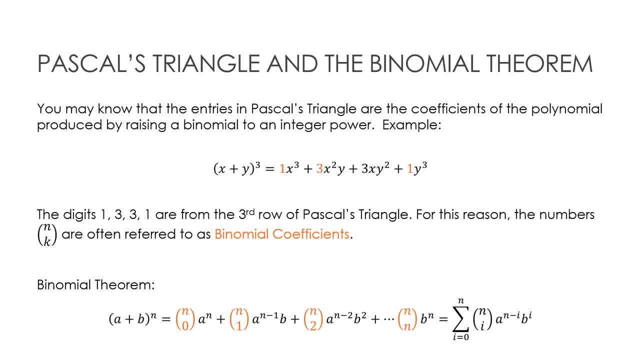 And we've talked about summation notation. but why? Why did we talk about summation notation? It doesn't seem to fit. Well, let's put it all together. Let's say I have a binomial, binomial being that I have two values being added or subtracted. 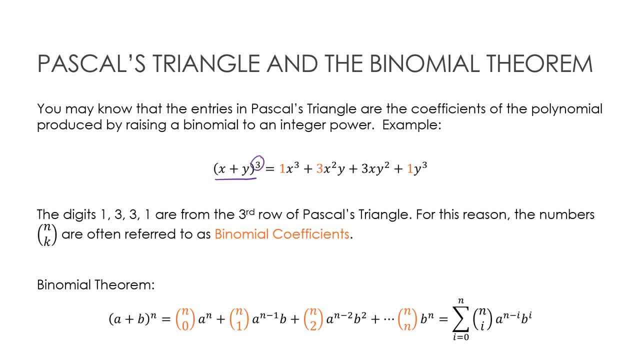 So I do have a peak position. The point is that my sine of p- So I have superfluous cosine of p- squared, And then I then have an integer of y. This allowed me to take one of these things. So I take x to the third, the second one, the first one. 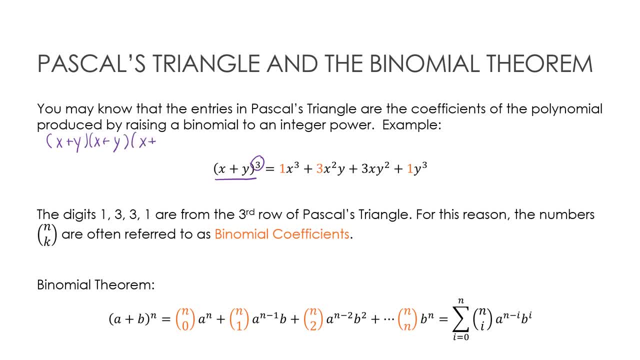 And then I multiply y times y to get x squared times y squared to the third. So I give a function, x squared times x squared, and then I multiply it to the third. Hopefully this works Okay. so now let's take x squared, minus my Latin. 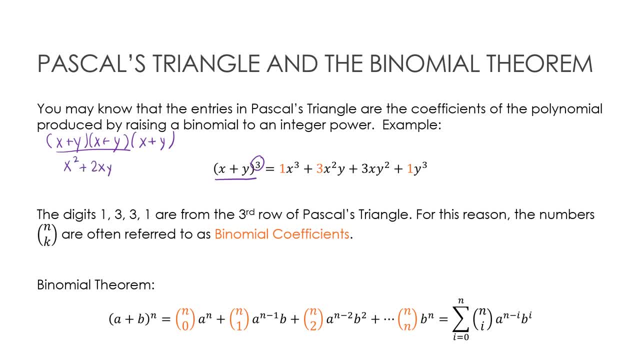 I'm bombs. at this point It works pretty smoothly. I take raise to some integer power. You could imagine an x to the third is amazing, though you might not realize it in person, because here I've showed you where the x is right now. 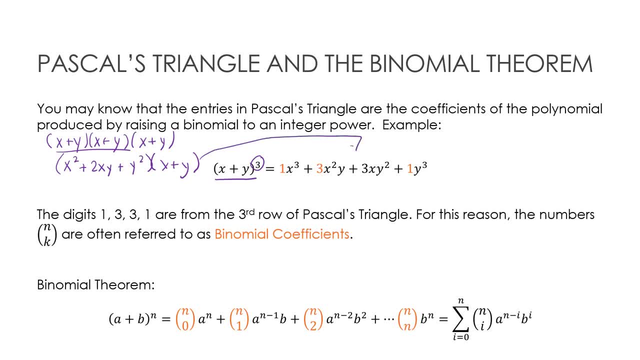 You can maybe use what you call the integral of the integral 1dx, and when I multiplied this out, I would end up here: 1x cubed plus 3x squared y plus 3xy squared plus 1y cubed. Now, why do I care? Why is that important to me? Well, let's take a look at 1. 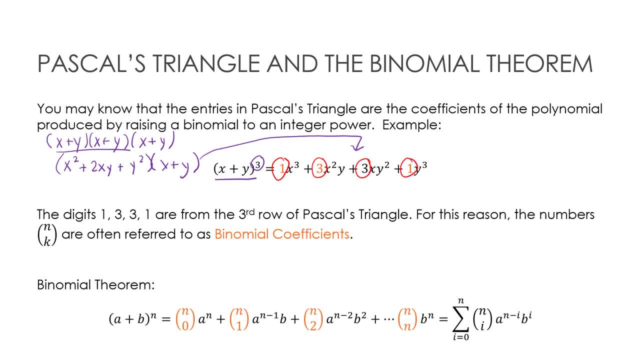 and 3 and 3 and 1.. Those digits, if you'll remember, are from the third row of Pascal's triangle. So, remember, I had 1,, then I had 1 and 1,, and then I had 1,, 2,, 1,, and then I had 1,, 3,, 3,, 1.. 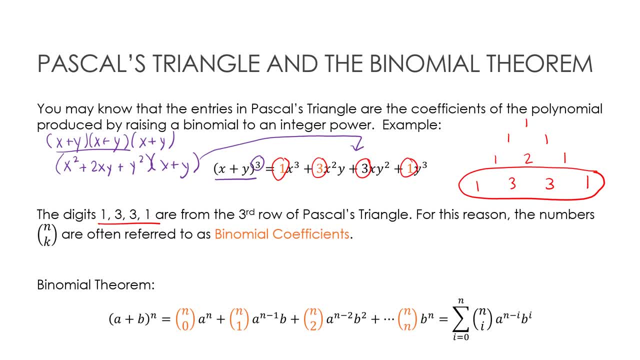 Those numbers are the same as what I just used in my answer. So for that reason, the number n choose k, because, if you'll remember, this was 3 choose 0,, 3 choose 1,, 3 choose 2,, 3 choose 3.. 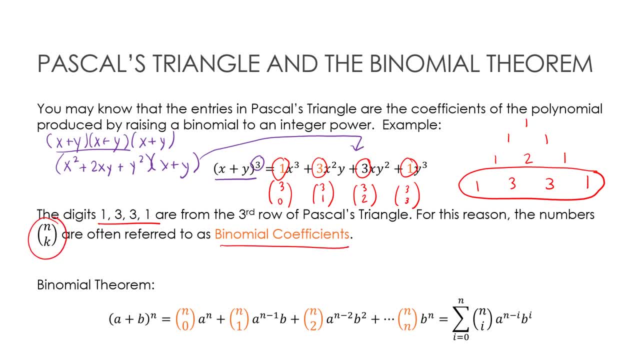 So I'm going to use this as my answer. So I'm going to use this as my answer. So n choose k. are often referred to as binomial coefficients. So the binomial theorem says that if you have a binomial raised to an integer power, that it's going to follow this format. 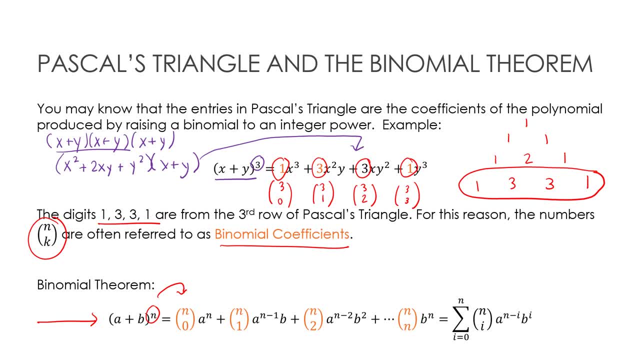 where I'm taking n choose 0, a to the n and notice that held true. here, n choose 1,. I'm going to decrease the binomial coefficients, So I'm going to take n choose 0, a to the n and notice that held true. 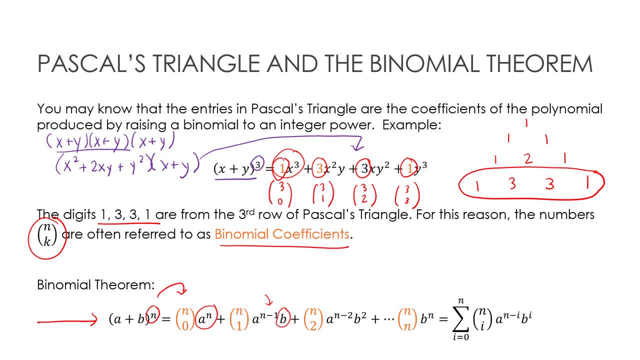 here n choose 1, a to the n and notice that held true. here n choose 1, a to the n and notice that held true. here a exponent by 1,. I'm going to increase the b exponent by 2, because essentially this was b. 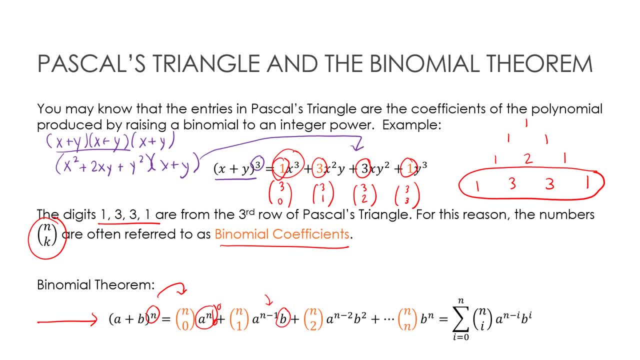 choose 0,, I'm sorry, b to the 0. And then that pattern is going to continue: this goes down one, this goes up one, etc. etc, etc, all the way until the end where I'm going to have a to the 0,, b to the n. 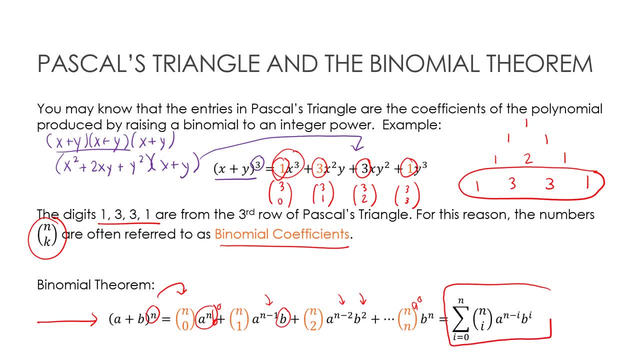 Now why did we review summation notation? Because that can be simplified into this. So the binomial theorem is often written as this: this equals this, which is to say the summation from 0 to n of n. choose i, so i is the value. 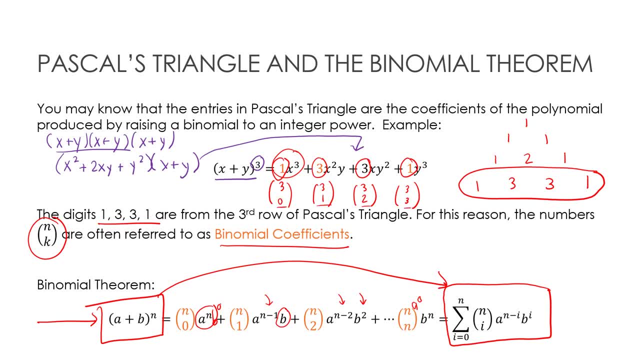 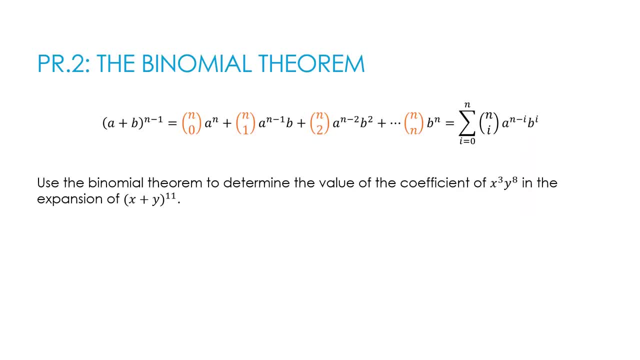 that's going to change 0,, 1,, 2,, 3, etc. of a to the n minus i, b to the i. So we'll see a lot more applications of this further down the road, but one application we'll use immediately will be a question like this, where it says: use the binomial theorem. 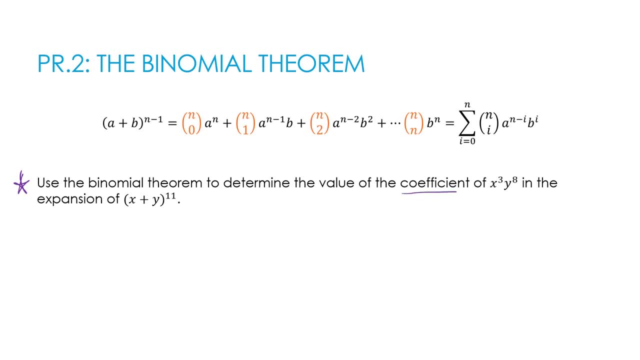 to determine the value of the coefficient- coefficient, of course, being what's the number that's going to go in front, of x to the third, y to the eighth. Now, what I would not want to do is to take, because there's obviously 11 total. what I would not want to do 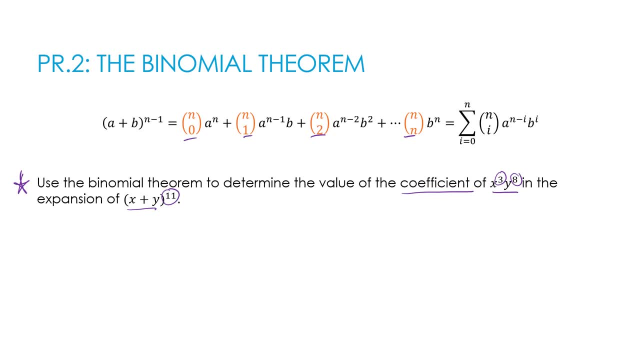 is actually: multiply x plus y out to the 11th, because that would be a lot of work for something that I don't need to show all of that work for. So instead, what I can do is I can say: well, I have 11. 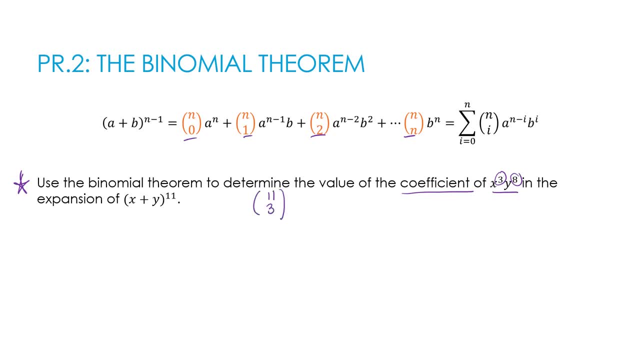 and I'm going to choose 3, or I have 11 and I'm going to choose 8.. Now, how can I do that? Well, because of that theorem we talked about before that says n choose k is the same as n choose a. 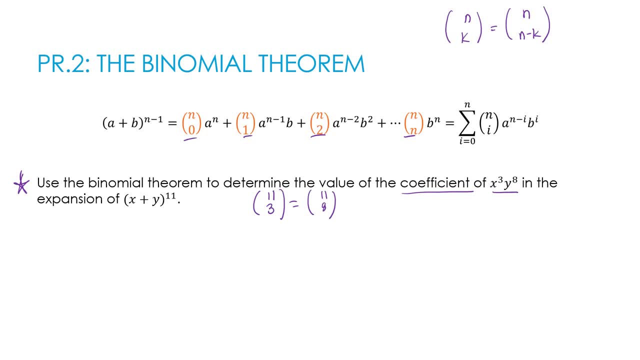 n minus k, And I know 3 and 8 are my two numbers, because those are the two numbers here and of course those add up to 11. So then I can just get my calculator out to compute what that is, and that's 165.. 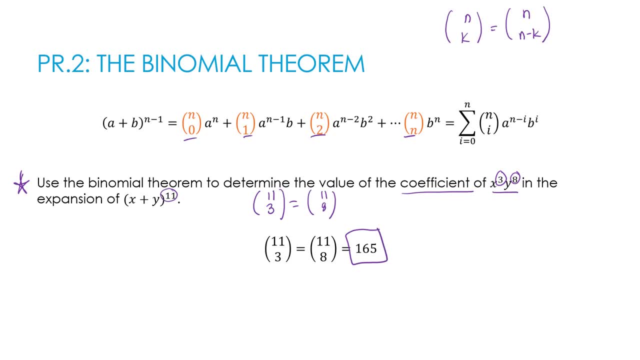 So what does that tell me? That tells me, if I were to take the time to multiply x plus y, x plus y, blah, blah, blah, x plus y, 11 total, If I took the time to FOIL those numbers, I would have a total of 16.. 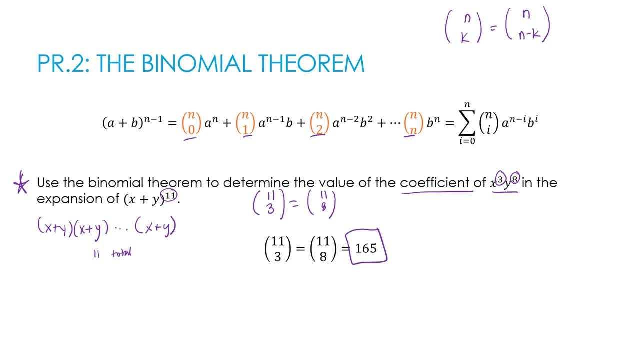 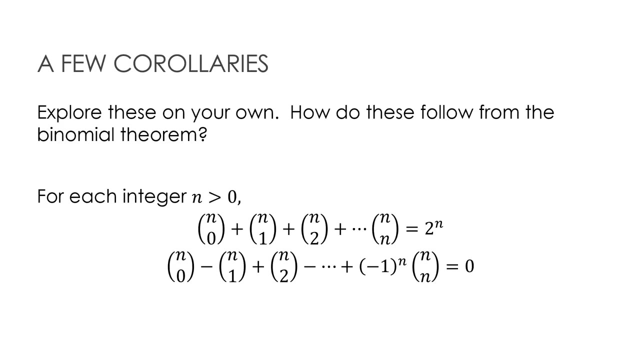 If I FOIL those out, combine like terms, FOIL it out again, combine like terms, etc. the term that included x cubed y to the 8th would have a positive 165 in front of it, And then I could continue to find those values. 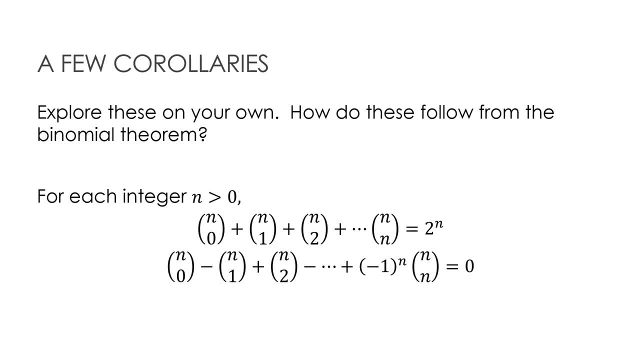 So here are a few corollaries, and I would encourage you to look at them both in detail, Particularly the first one. You might see it again, But how does the binomial theorem that we just talked about lead us to this? So I'm not going to go through that with you. 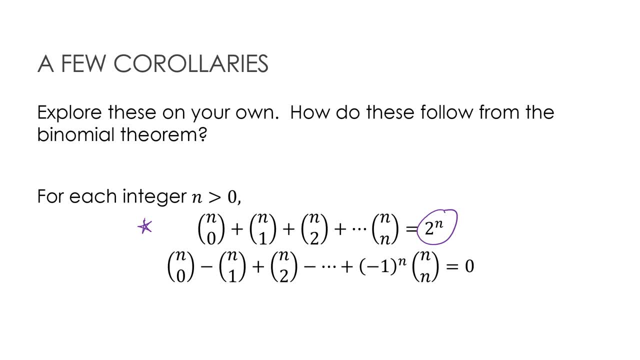 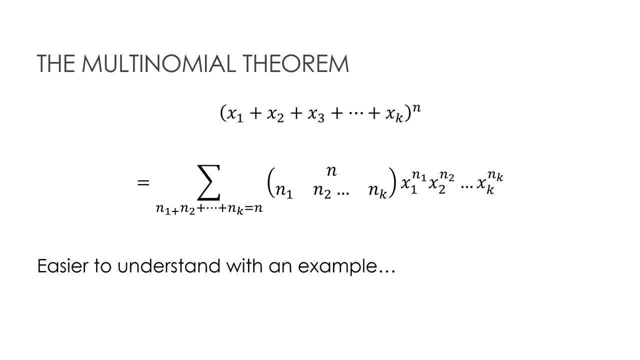 I believe it's in your textbook. If not, obviously you may Google, But I want you to actually struggle with it a little bit before you just Google to find the answer. We're going to finish out with the multinomial theorem, and that essentially is for when. 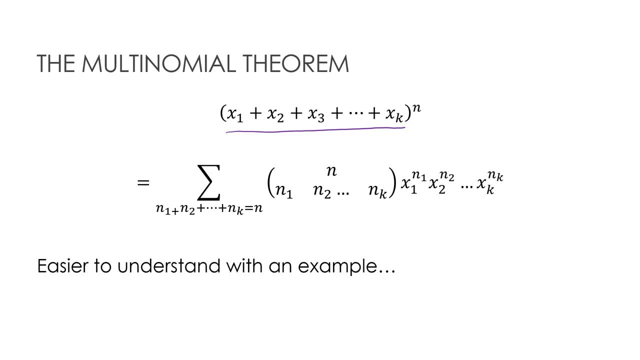 we don't have a binomial, but we have several values that are being integrated. They are not going to be added or subtracted, taken to an integer power. Now this guy looks like a hot mess, And so I don't even want to really explain it to you until I can show you an example. 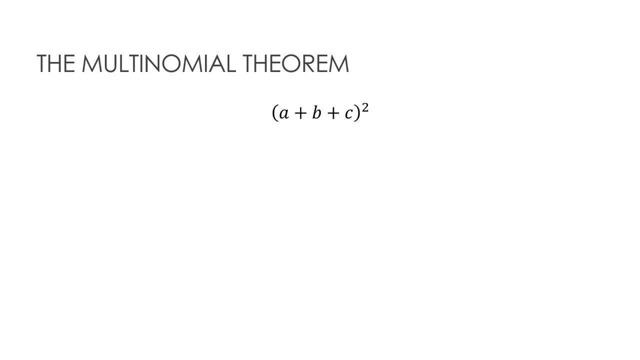 So let's just put this on hold for just a moment and go look at the example together. So let's take a look at this example. If I didn't give you the multinomial theorem, we would just have to plug and chug through. 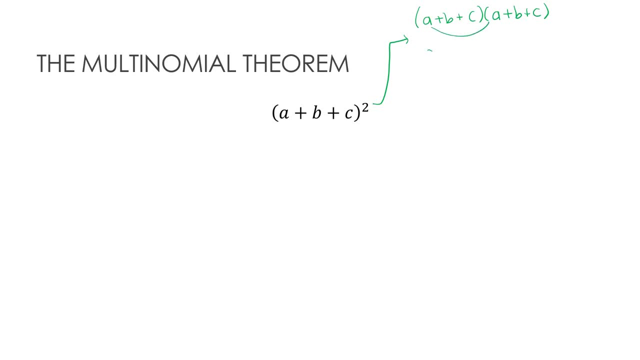 this plus b, plus c, and we know it's pretty straightforward. it's just that it's going to take a while and that's just the a's, and then i would have to do the b's, then i would have to do the c's, then i would have to combine like terms now for something that was squared like this: this one. 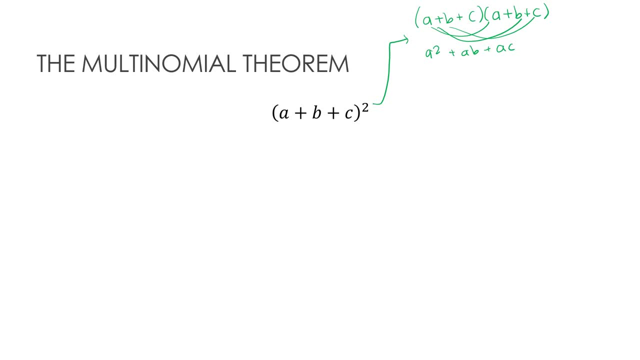 actually might be shorter, but let's take a look at what the multinomial theorem will help us to do. so this would be our first line of work. and don't freak out yet, because here's what all of this means. i know that i'm going to have some value a squared and then some value b squared, and then 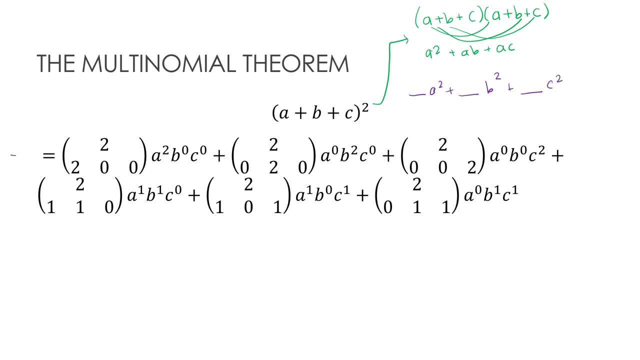 some value c squared. that's this first row. and where do i get the numbers? well, this is the multinomial theorem that says: n is 2 and i'm choosing n is 2 and i'm choosing 2, choose 2 a's, 2, choose 2 b's, 2, choose 2 c's. and notice that corresponds to how many a's, b's and c's i have. 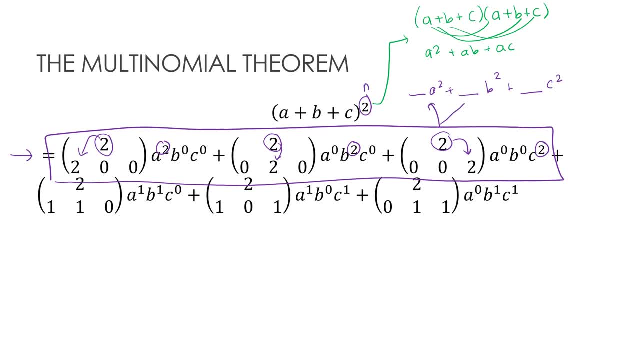 so essentially, that would give me these fill in the blank options. then i know that, in addition to those, i'm going to have something a- b, i'm going to have something a- c and i'm going to have something b- c. and how do i get that again? that's these guys. 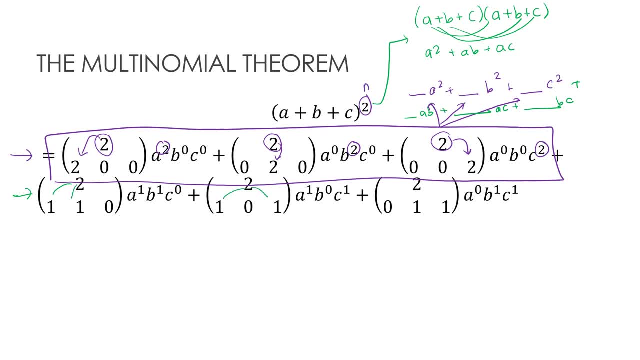 so 1 a, 1 b, 1 a, 1 c, 1 b, 1 c. what do those by our multinomial coefficients turn into? well, essentially, what we're saying is: take 2 factorial over 2 factorial, 0 factorial, 0 factorial. same thing here: 2 factorial, 0 factorial, 2 factorial. keep in mind that 0 factorial is 1. 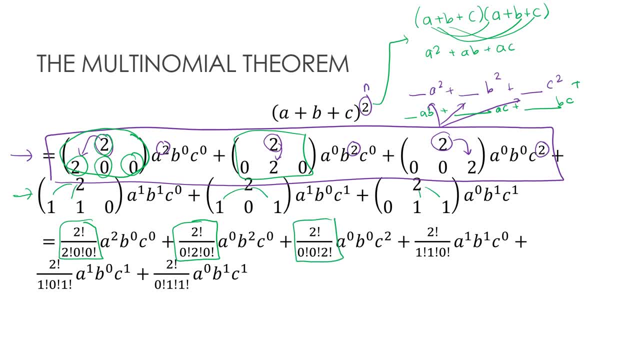 and then that's for the third, and then for the next line: 2 choose 1, choose 1. 2- choose 1, choose 0, choose 1, 2 choose 0, choose 1, choose 1. and then use your calculator: a squared, because 2 factorial over 2 factorial is 1, so a squared plus b squared plus c squared. 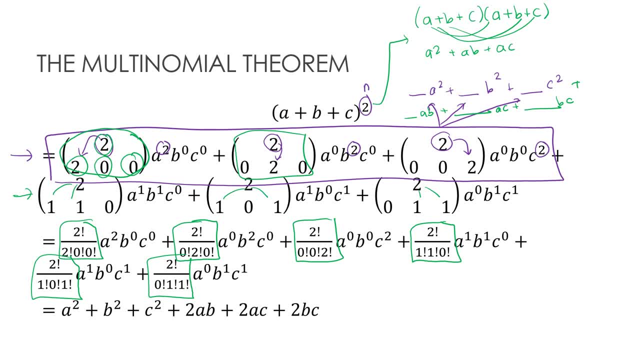 and then 2 a b, 2 a c, 2 b c, and if you don't believe me, please feel free to multiply this out and to determine the final solution, but you should end up with what we ended up with here. you.